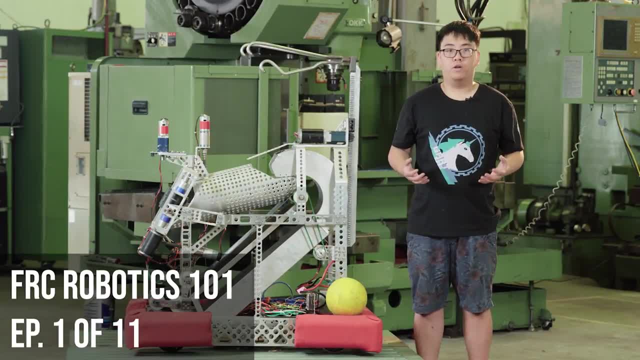 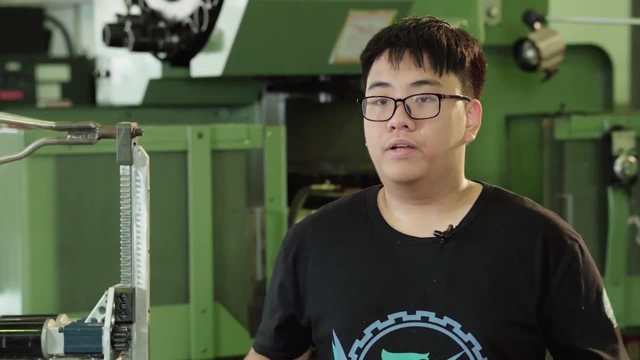 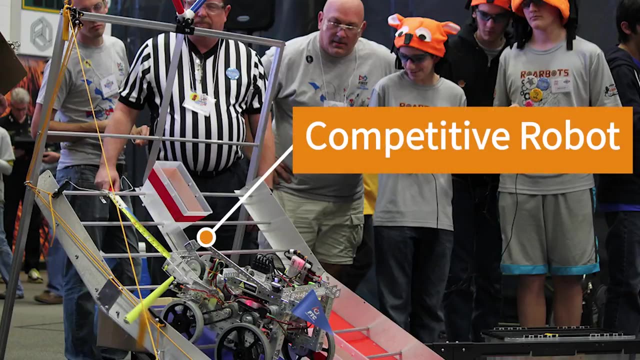 Hi, welcome to the first episode of FRC Robotics 101.. I'm Thang and we're from FRC team 6520, Green Amps Robotics team. This series, as follows, will be dedicated to the process of making a competitive robot based on our experience in the FRC. So this series will be geared toward people who want to. 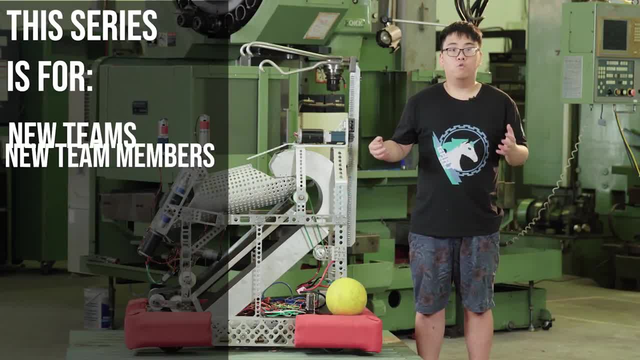 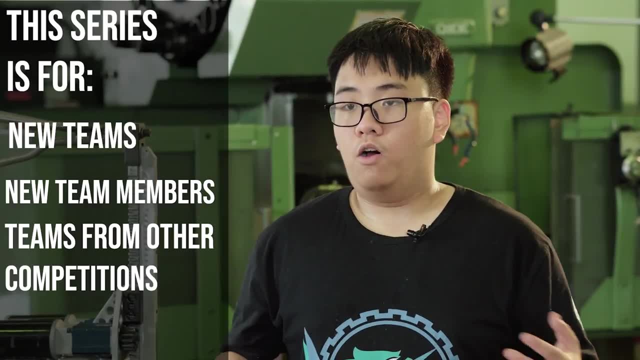 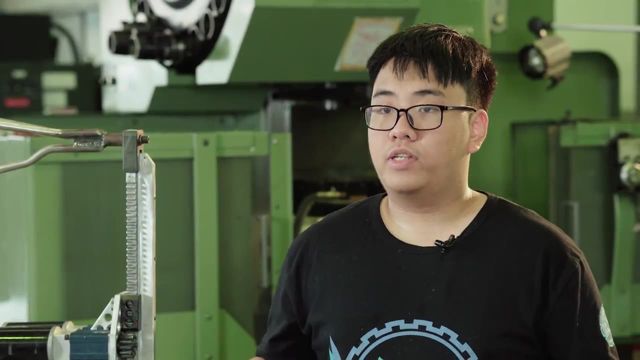 set up a new FRC team or just new members who want to know what's ahead of them. If you are a student who is related to a non-FIRST project, you are also welcome, as this can serve as a general skeleton to whatever creative process you're doing. In this first episode, we're just going to go through what 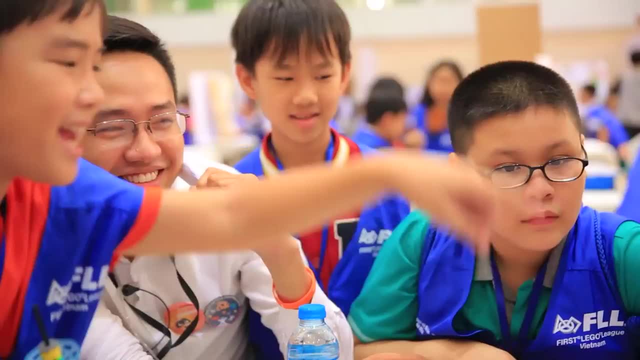 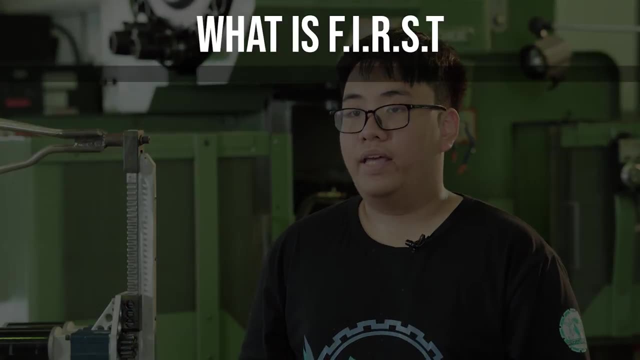 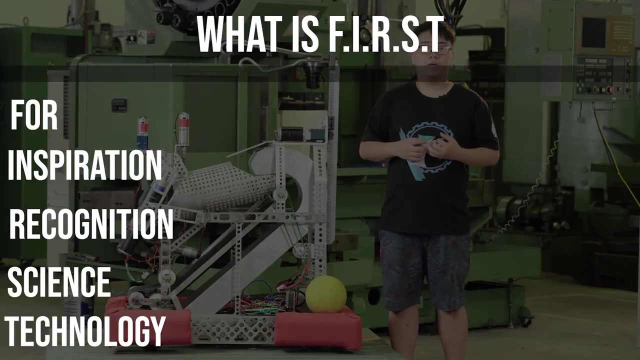 is FIRST- how to organize your FRC team, and we're going to go in-depth about two specific departments: the Mechanics department and the CAD department. So let's first talk about FIRST. FIRST stands for for Inspire- Inspiration and recognition of science and technology. FIRST is an international organization. 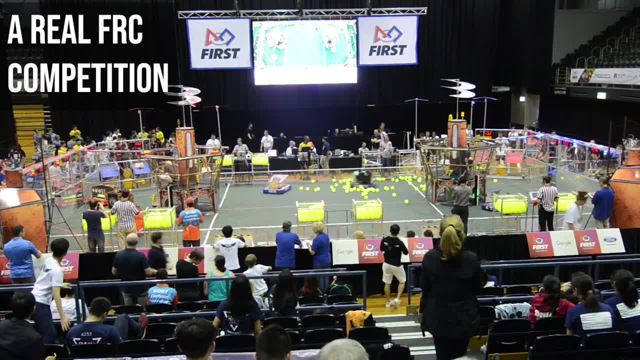 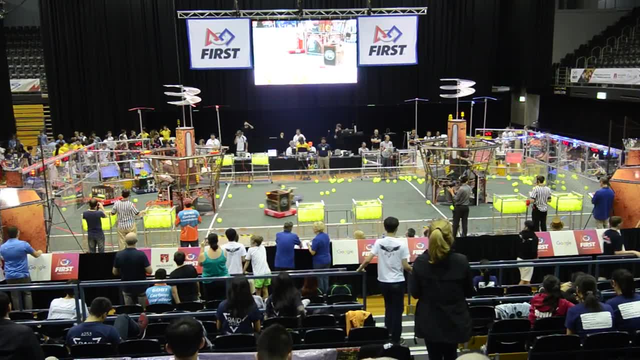 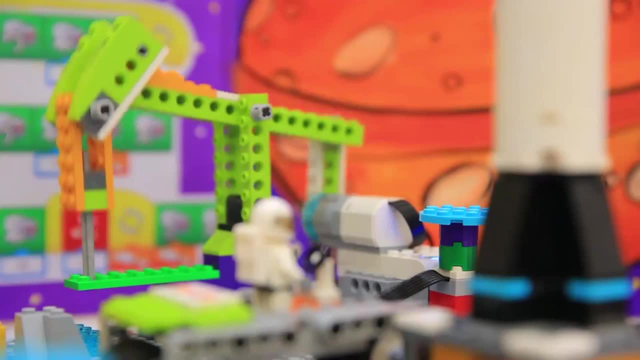 that organizes many different robotics competitions, Their biggest competition being the FRC. that is a robotic competition for high school students. For younger audiences, they have the FIRST LEGO League Junior, the FIRST LEGO League and the FIRST Tech Challenge. Just recently they started the FIRST Global, which is a competition for representatives. 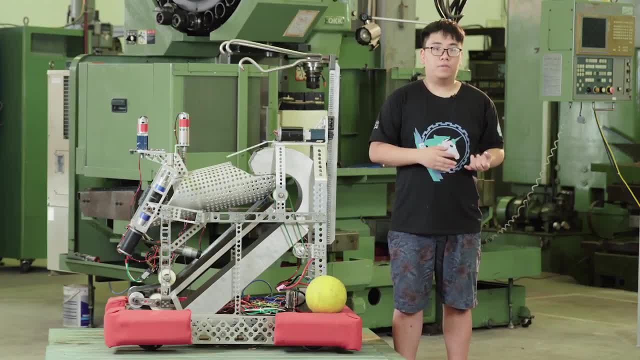 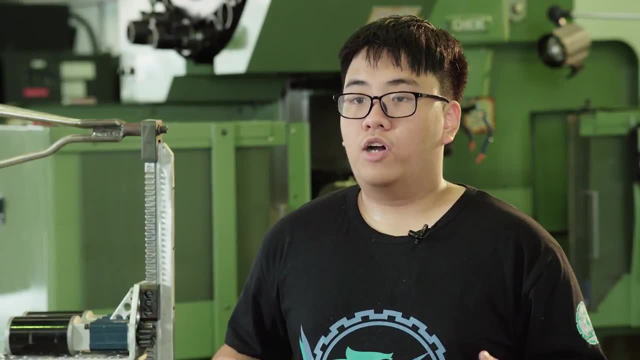 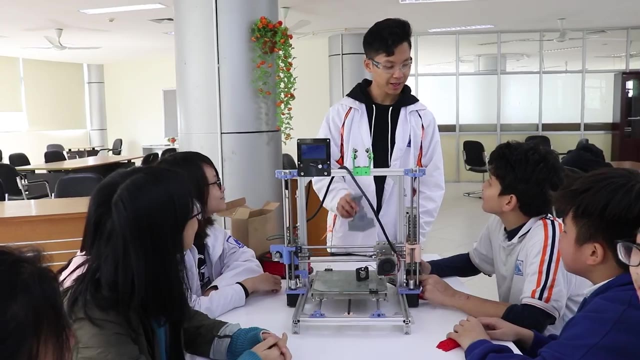 from all over the world to compete in a competition that is smaller scale than the FRC. Now let's go in-depth about the FRC. The FRC is the largest annual robotics competition for high school students. It provides high school students with hands-on experience about 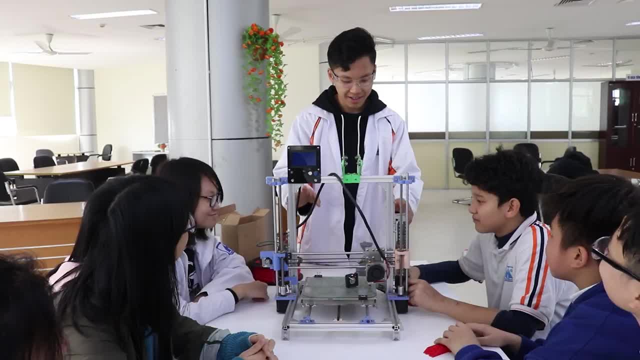 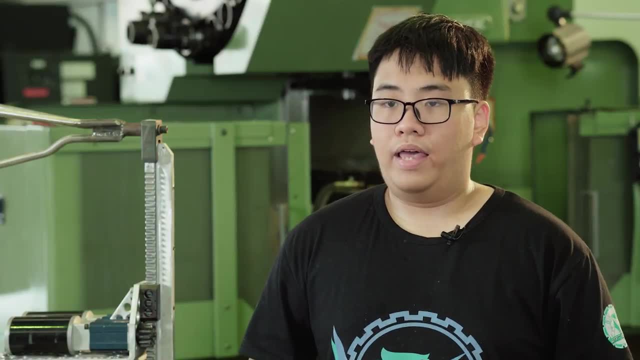 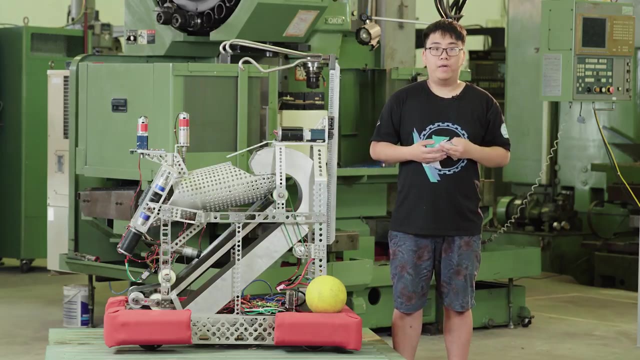 many different technical skills like programming, mechanics, CADing and many more. You also get the experience of managing a huge team. An FRC season will consist of three main parts. First is the off-season, that is, the preparation and research and basically everything that you. 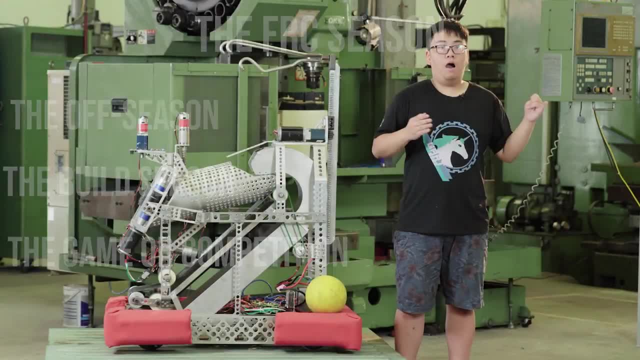 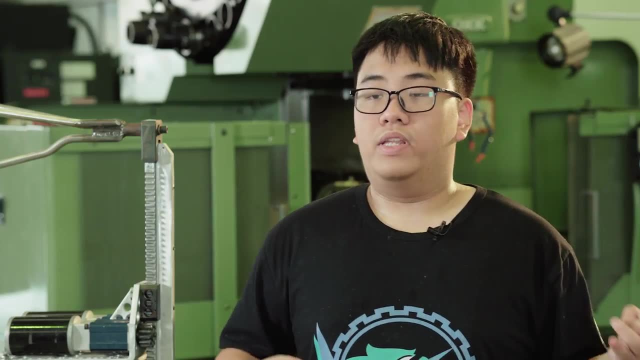 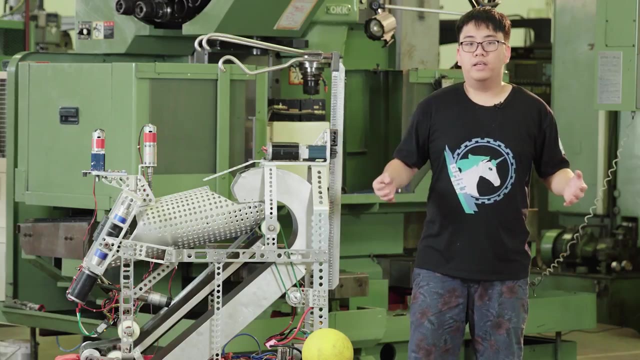 need to do to train new members, to prepare for your robot, anything that is before your actual season- Then when you're given the game manual on the 5th of January, then it will be the build season. The build season is the part where every member on the team has to work intensively to build the 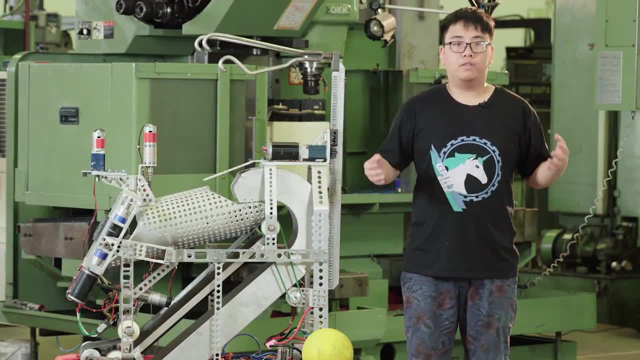 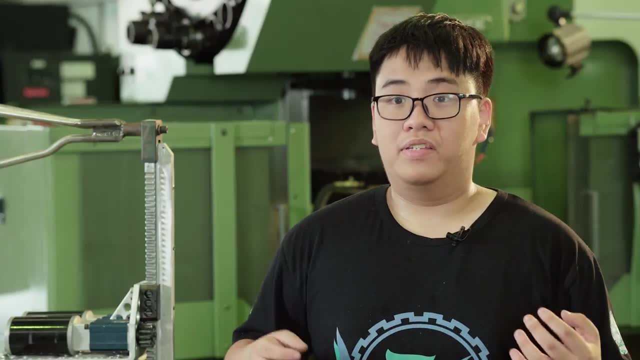 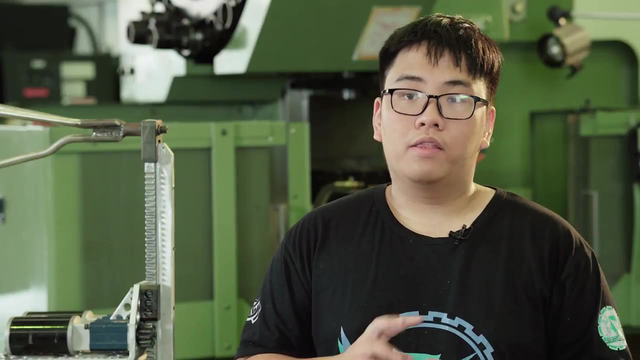 best robot they can and compete for many different awards And lastly, you have the actual game. The actual game is like its name. when you go to the actual competition and compete, There are two main rounds- the regionals, and if you win the regionals or get enough awards, you can go to the. 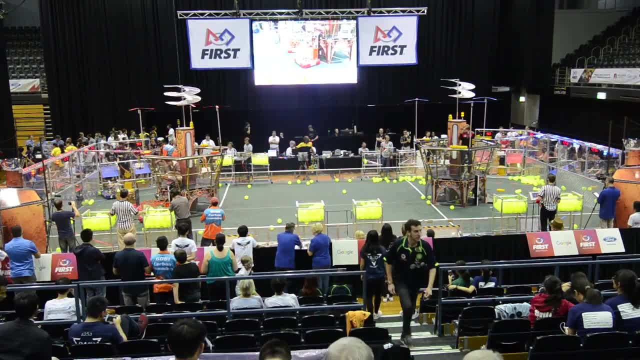 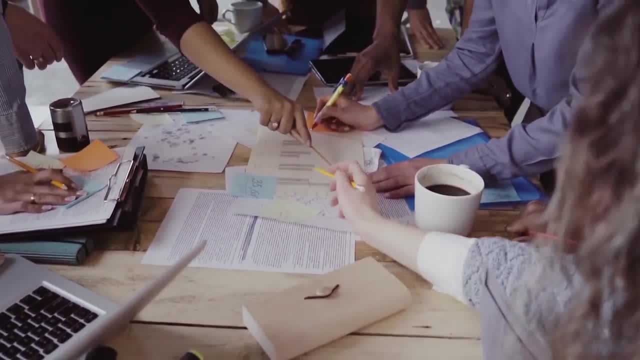 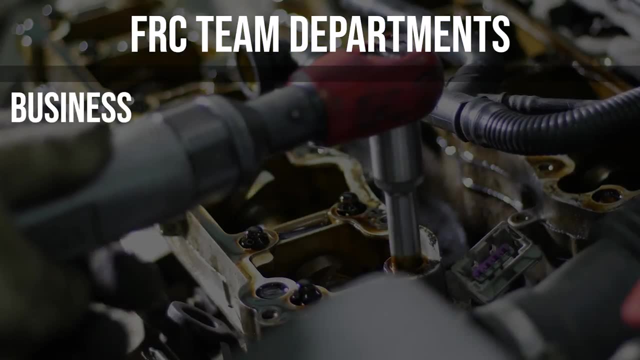 regionals and get the best robot you can. Each one of those will consist of a qualification round and then a playoff. Now let's get into how to actually organize your FRC team. An FRC team will consist of many different departments, from business to outreach, to mechanics and electronics. 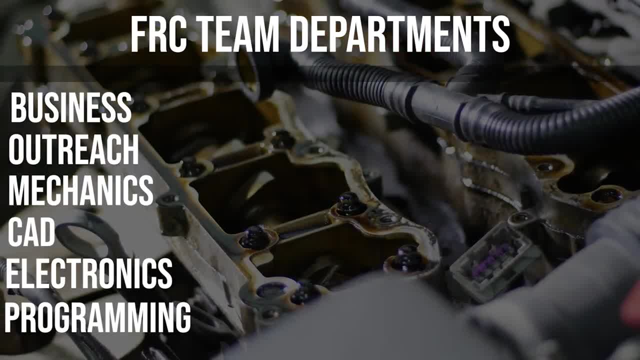 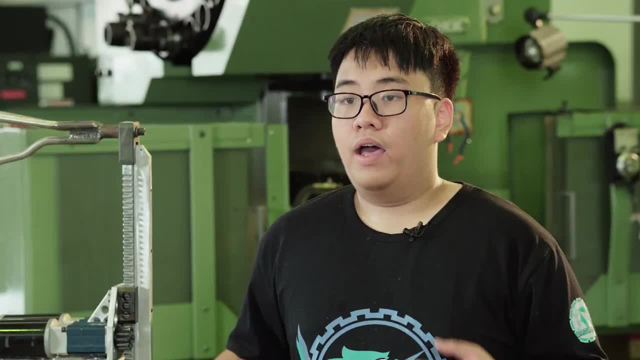 and also many more. Teams need to be separated into different departments to work as efficiently as possible, And also because one member can't learn to work on their own, they have to be separated into different departments to work as efficiently as possible As a team grows. 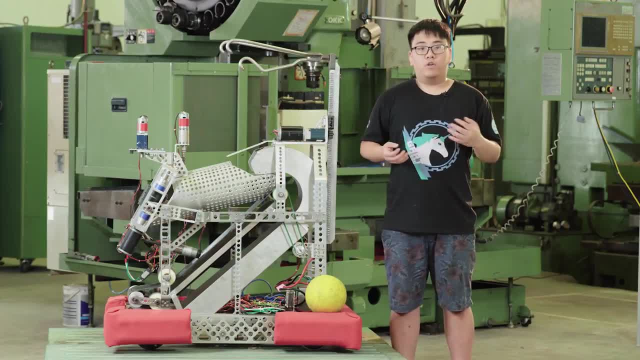 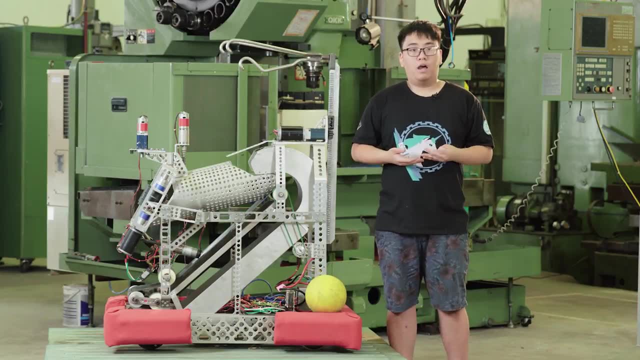 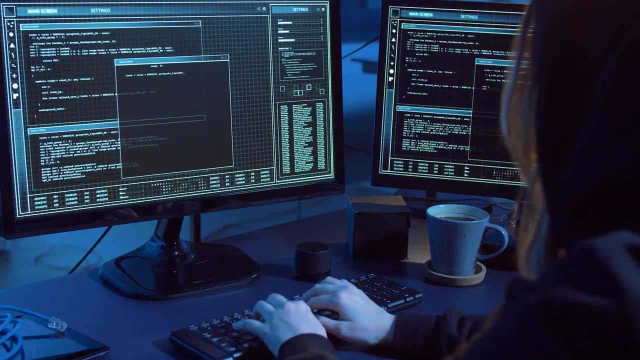 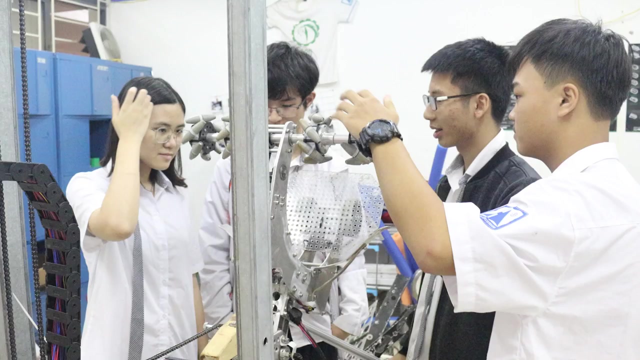 departments will be divided even more. For example, the programming department can be divided into pathfinding department and then vision department. You can also do the same for many other departments. For now we can just go in depth about two specific departments, As we said before: the mechanics department and the CAD department. So 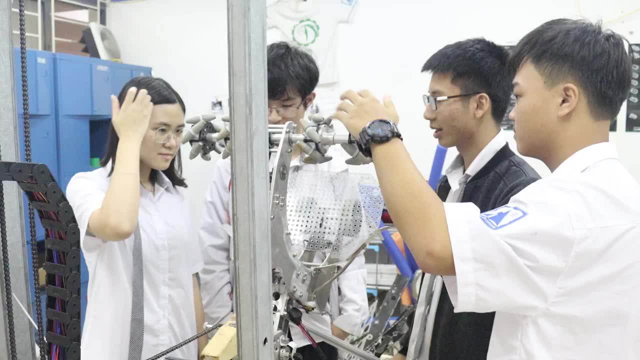 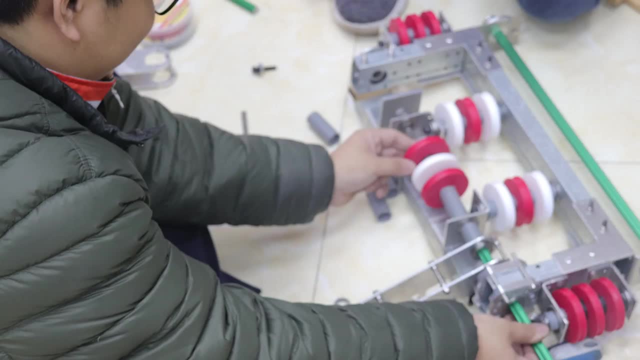 first let's talk about the mechanics department. The mechanics department is the department that has everything to do with building the robot and constructing the field. Their job. their work is evident in many different places. Anywhere you look on the robot, that is their work. 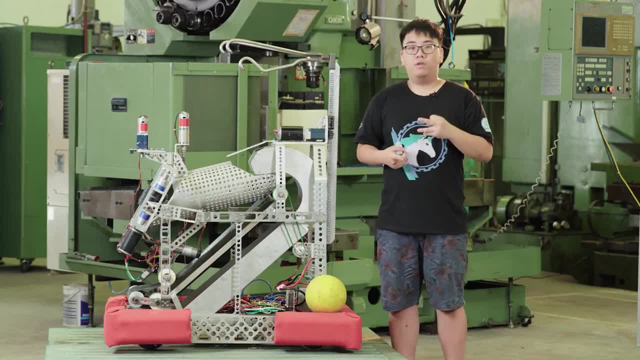 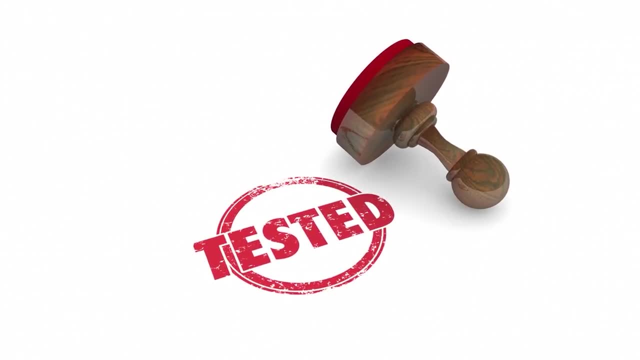 They're responsible for building the robot, building the game field, reparation, maintenance and things like testing and tweaking the numbers. Basically, if you want something done, most likely it will be their work. Then you also have the CAD department. 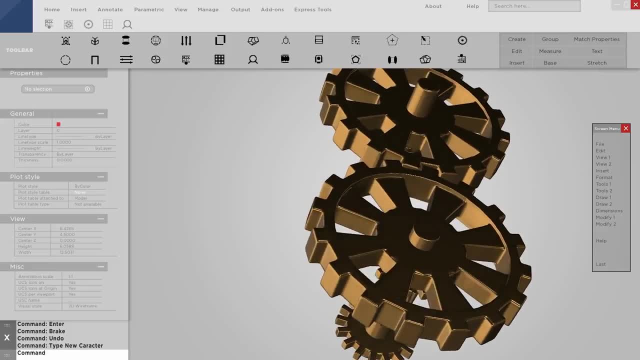 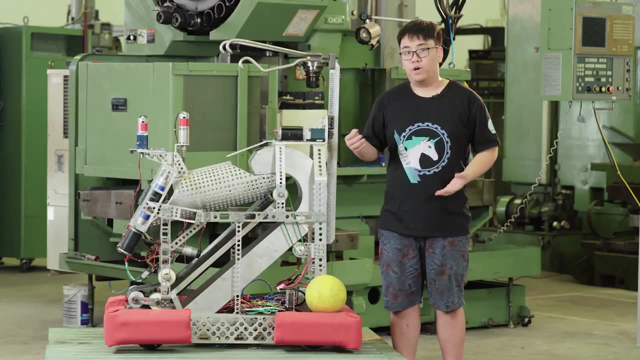 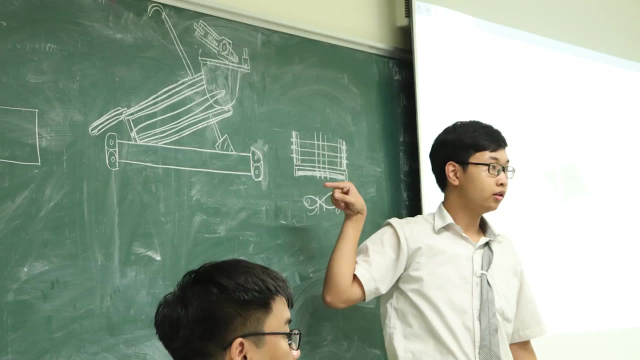 CAD stands for Computer Aided Design. The job of this department is to build the 3D and 2D model of whatever you're going to build for your final product. This 3D model is very useful in that if you change one number, the result is shown immediately. You don't have to spend a lot of time. 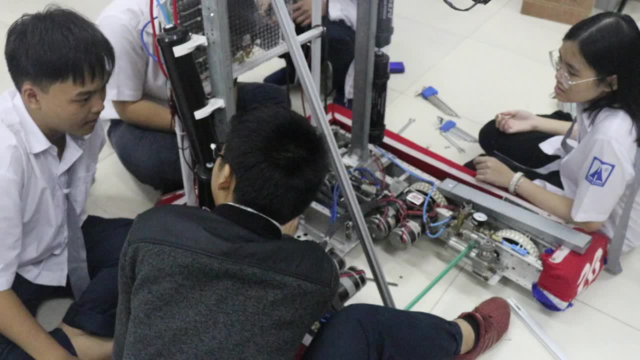 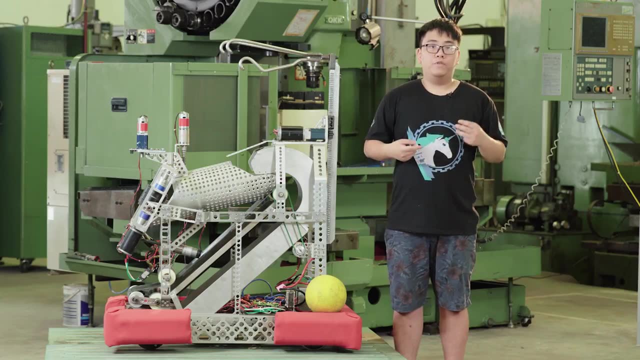 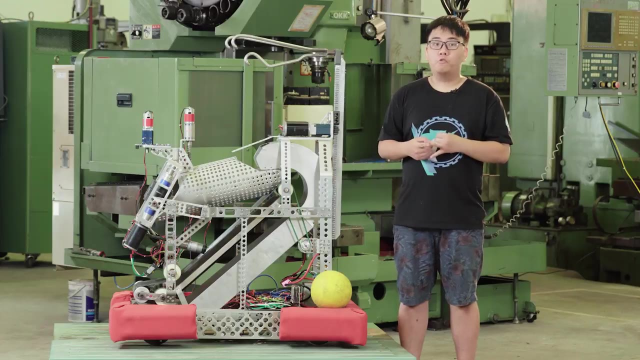 modifying your parts. You don't have to spend a lot of time working on it before seeing the result. Also, it is useful for calculations and just to visualize things, And your CAD file is necessary if you want to do CNC Next, since most people are familiar with things like mechanics or programming, but not as much. 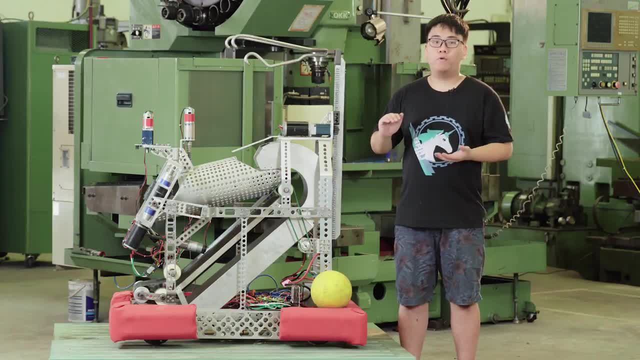 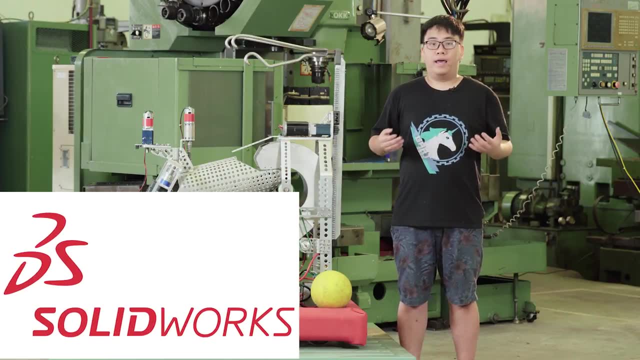 with computer-aided design. I just want to go through some programs that are often used when you're doing the FRC. The first CAD program is going to be SOLIDWORKS. SOLIDWORKS is a CAD program that is very robust. 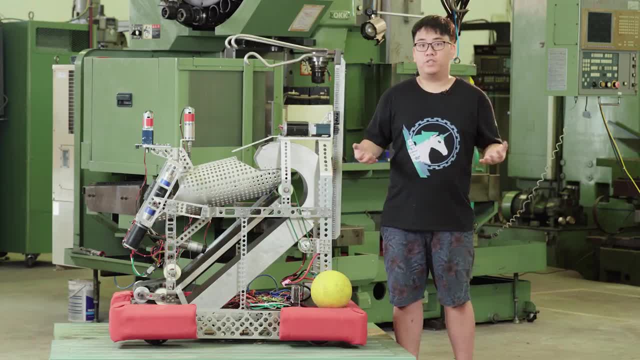 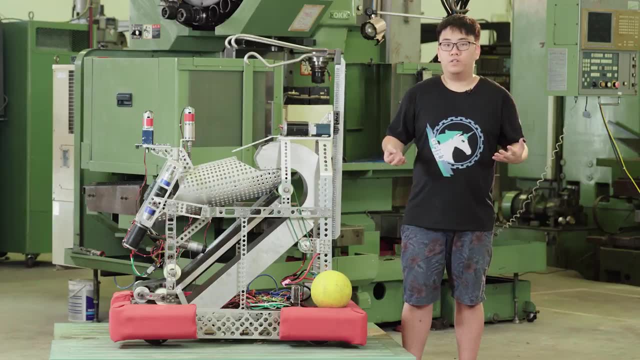 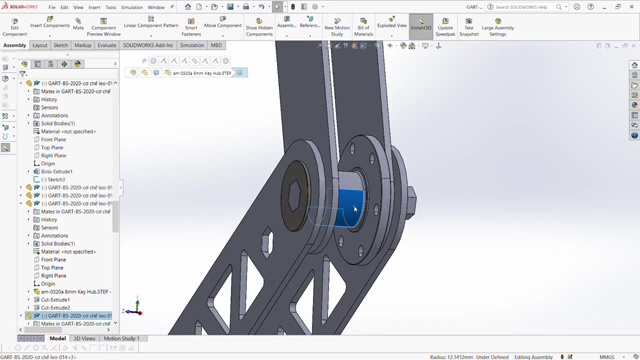 Normally it would cost quite a bit to get yourself a version of SOLIDWORKS, But because SOLIDWORKS sponsors the FRC, each team will get 50 versions of SOLIDWORKS each year, So that's why it is the most common for students doing the FRC. But if you're just starting out, or not related to 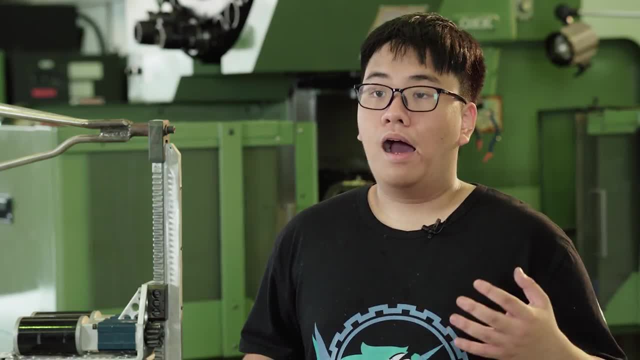 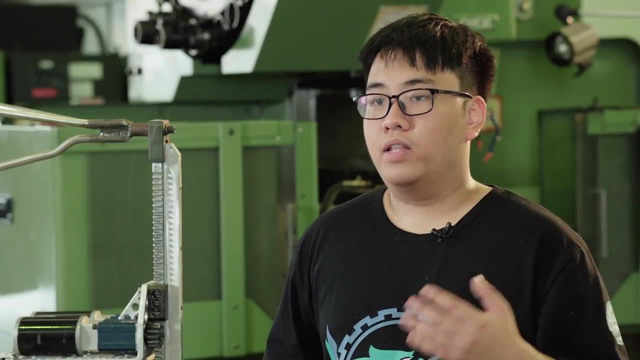 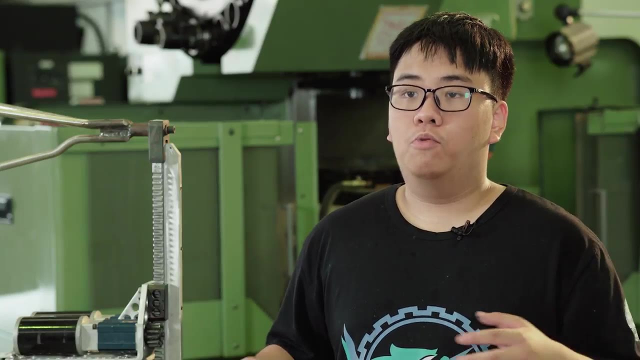 any FRC team, you might consider using Fusion 360.. Fusion 360 is a CAD program that is cloud-based, which makes it very light, So it's the perfect thing when you're just starting out. While it is not as robust, you can still do most of your tasks on Fusion 360.. 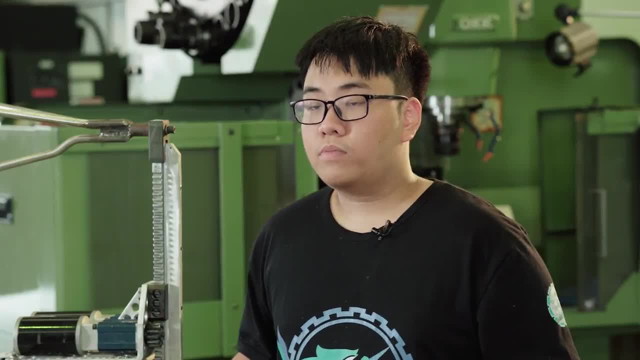 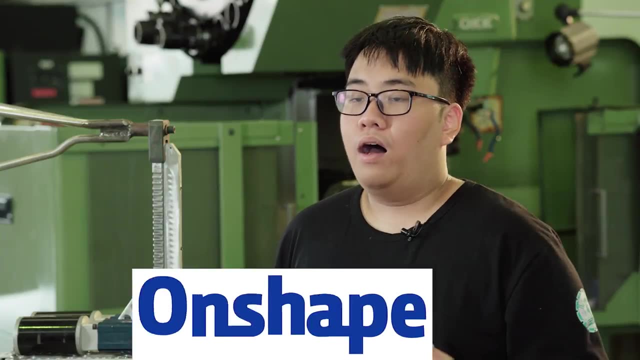 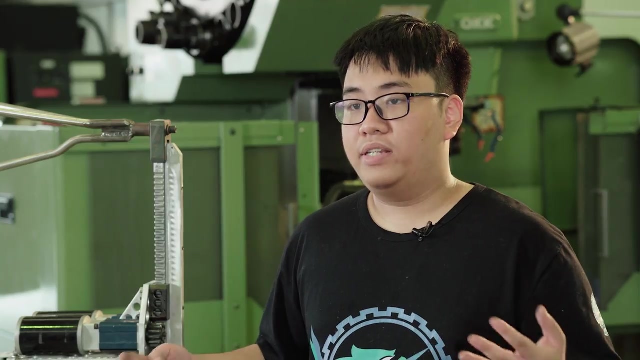 So it is the perfect one for new members. Then we can move on to Onshape. Onshape is a web-based CAD program. Being web-based means that you can access it from basically anywhere. You don't need your computer. You can even access it on your phone. But being web-based also means